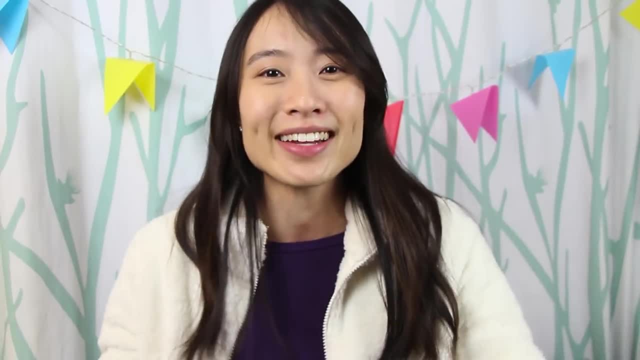 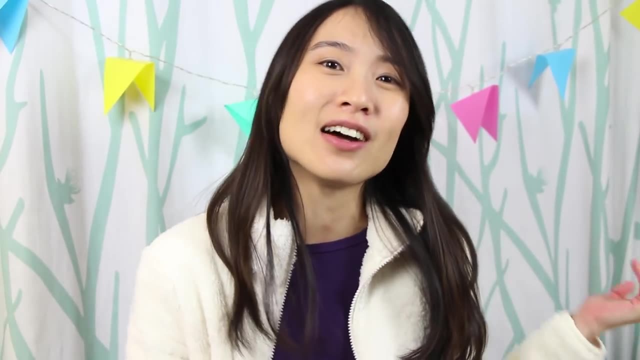 excited to share with you another year of crafty fun. If you are new to my channel, welcome, and be sure to hit that subscribe button along with the notification bell, so you'll be alerted of new crafty fun videos when they come out And without further ado. 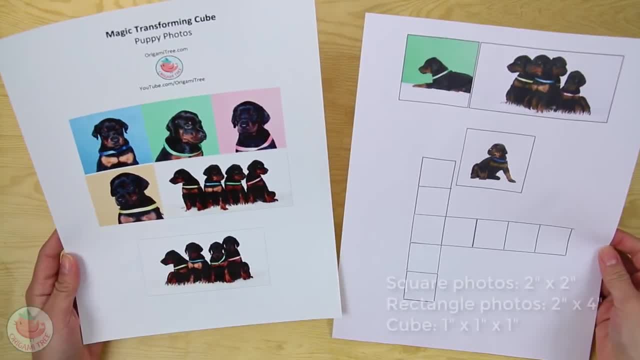 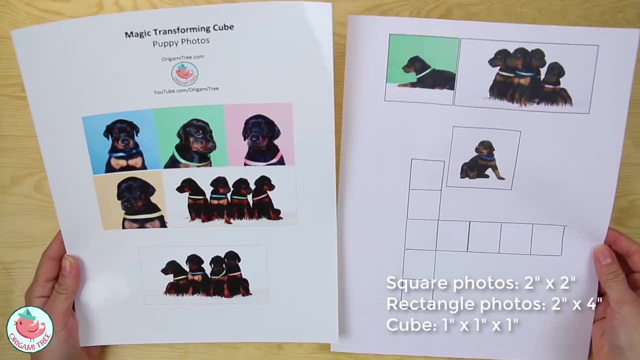 let's jump right in To make the transforming cube. you're going to start off by printing the template with the puppies and also the template for the cubes for my website. I'm going to link this to the video description below. It's going to have all the pictures. 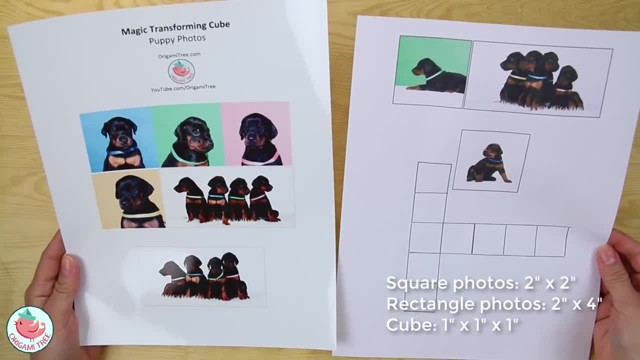 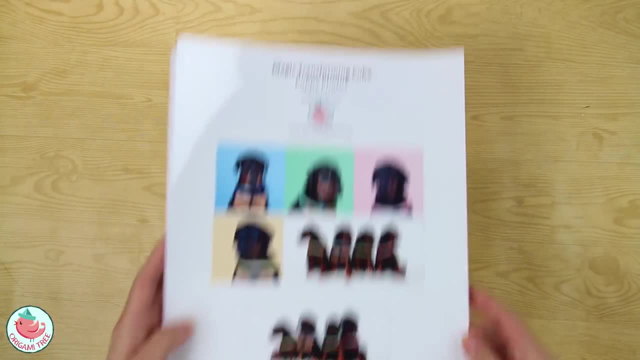 and everything you'll need to create this project. Now, if you don't have access to a printer or you don't own one, you can always create your own templates and photos as well, which is why I've written down the dimensions for you on this video. So, after you've printed, 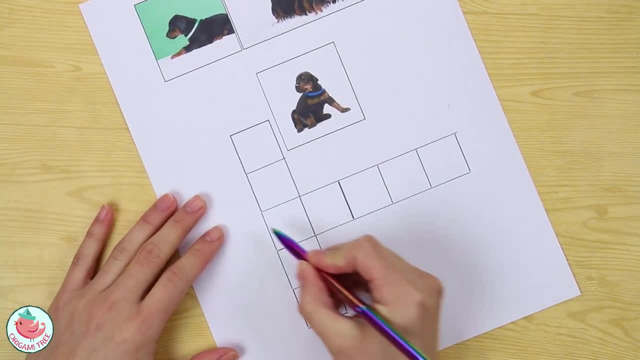 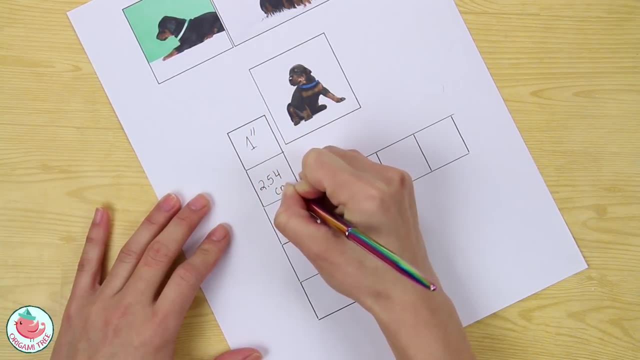 out the template. at the very bottom you'll see this T shape full of squares. Now these are 1 inch squares, or 2.54 centimeters If you use centimeters. Now let's take a pair of scissors and cut out the T shape. 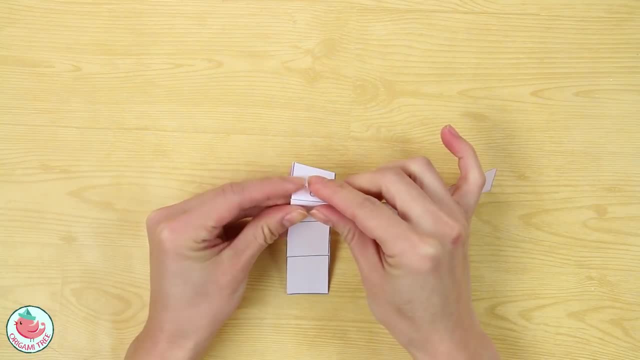 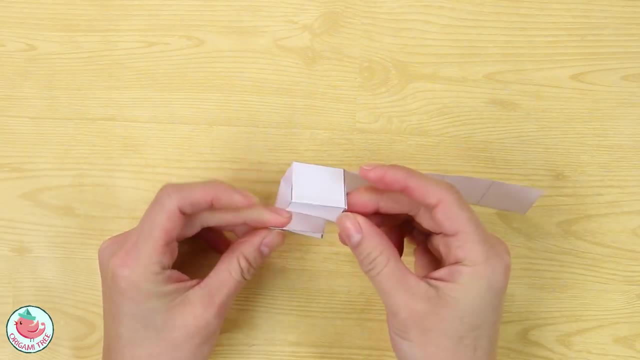 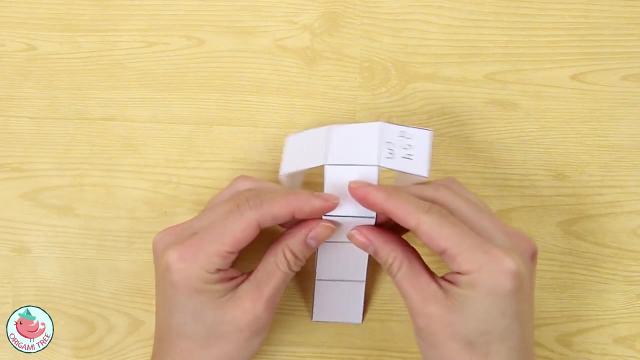 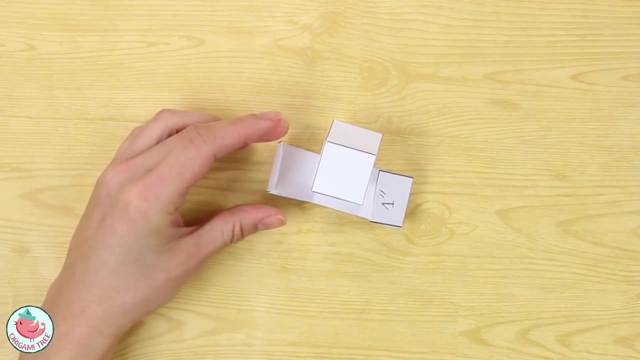 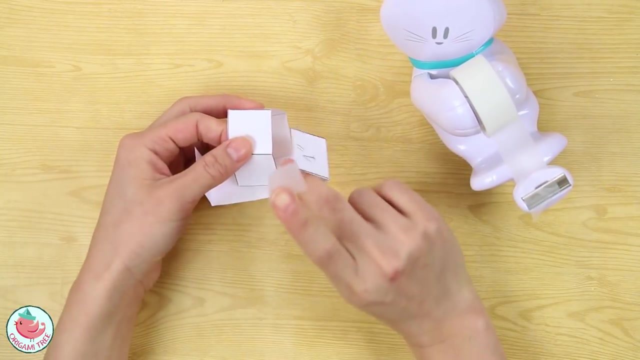 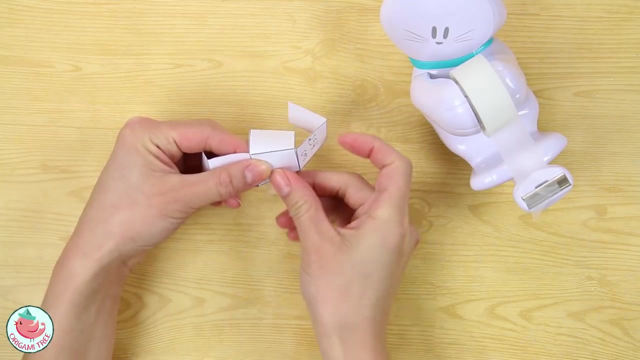 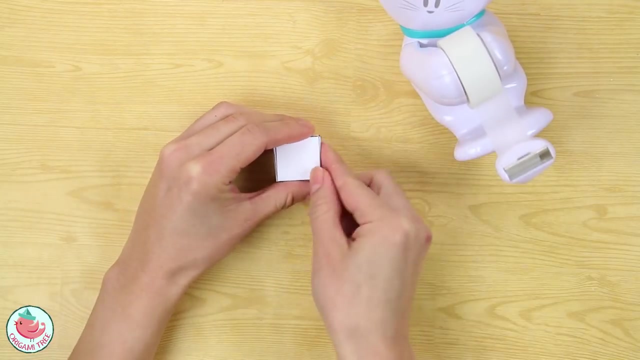 Once you have the T shape, you're just going to fold along the black solid lines, like I am doing here. Now the last part. the last part is the cutout. I'm gonna cut these out as well. So once you have all the creases made, you are now ready to assemble your cube. I'm just 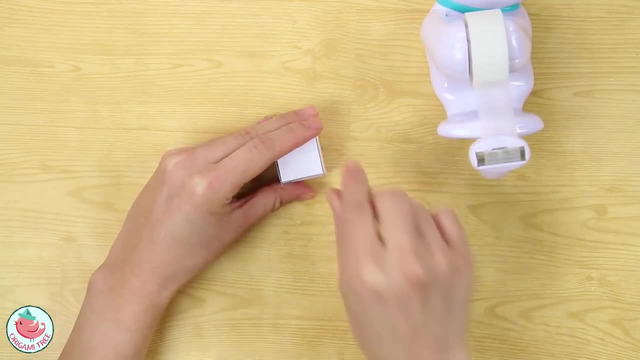 using clear tape by scotch, and this is my little kitty dispenser, which is really funny because this is a video about puppies. But anyway, you wrap the long edge of the T and then you're tape because you want to make sure that your cube is nice and sturdy. 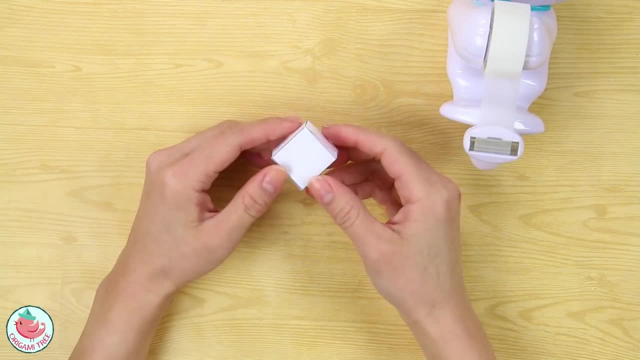 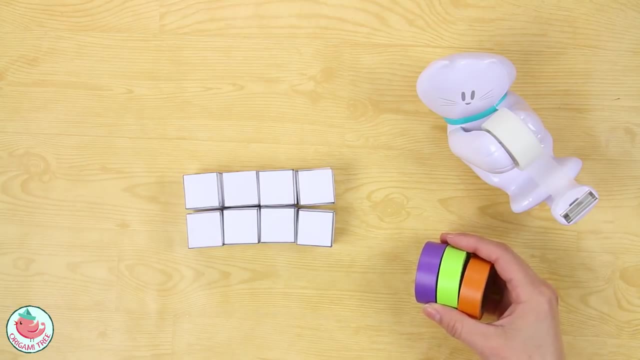 Once I've sealed all the sides with my tape, my first cube is completely done, and now you're just going to make seven more. This next part can get a little tricky, so I am using colorful washi tape- purple, green and orange- that I got from Paper Mart, and I will be using this as sort of a guideline of where to 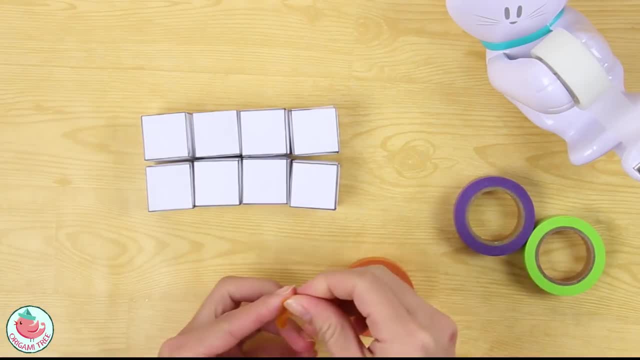 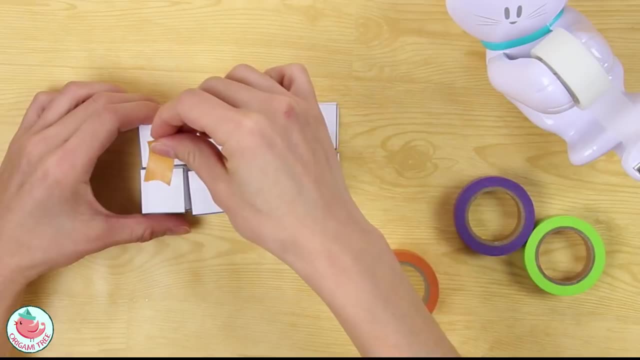 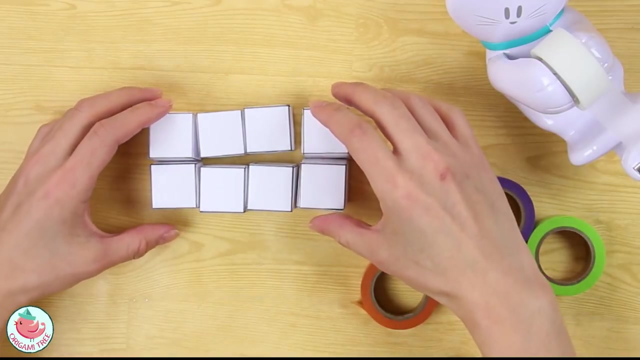 tape to seal everything. together With the orange washi tape, I'll be taping the far right cubes together and also the far left cubes together vertically. Now you want to flip the far right and far left cubes around where the orange tape is, and now you're going to be using your purple tape. 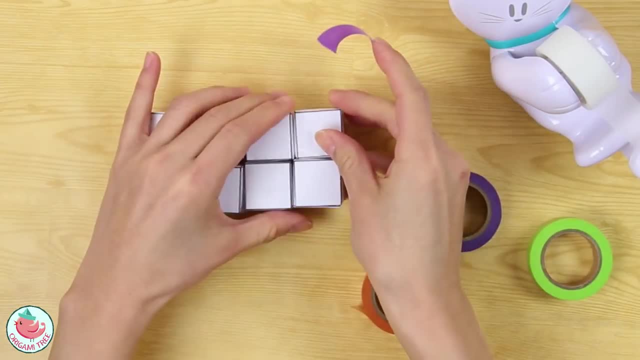 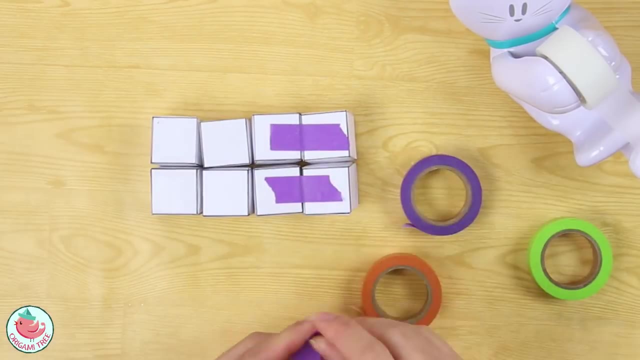 With the purple washi tape, I'll be taping the top two cubes on the top row, on the upper right hand corner, horizontally. Then I'm going to do the exact same thing underneath, and now I'm moving over to the upper left hand corner and I'm taping the top two. 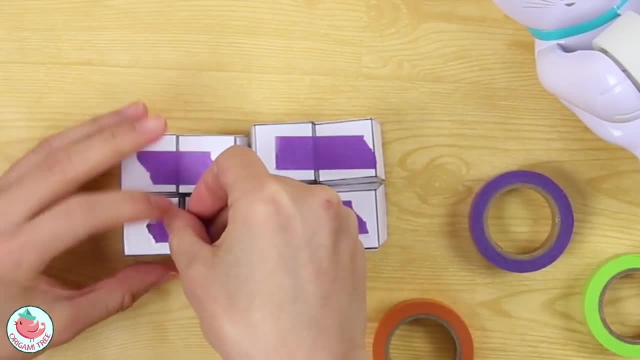 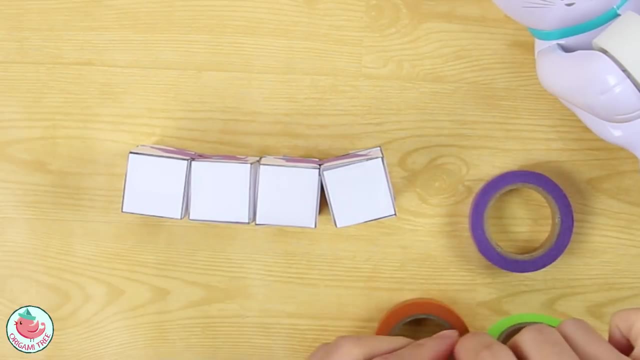 on the upper left hand corner horizontally and also doing the exact same thing right below it. Now I'm flipping the entire thing on the side and I'm going to take my green washi tape and I'm going to tape the middle two cubes together horizontally. 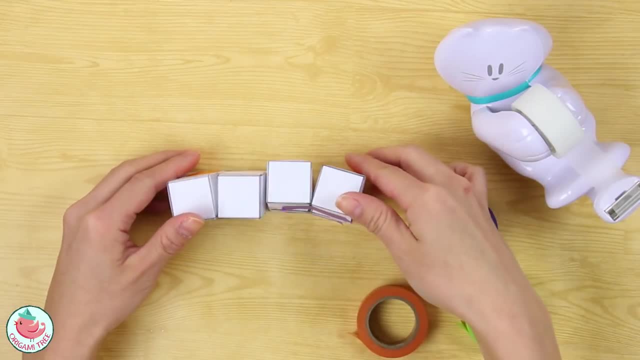 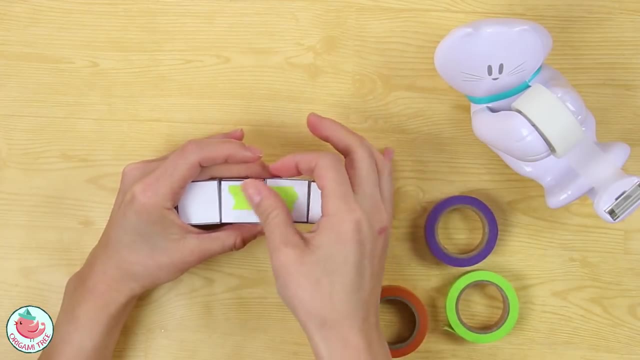 Now we're going to do the exact same thing on the other side, so you flip two times and then you're going to flip the center cube and you're going to tape the top two cubes together And then, using my green washi tape, I'm going to tape the two center cubes together. 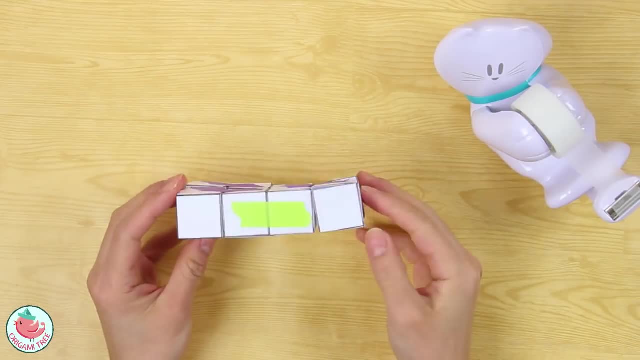 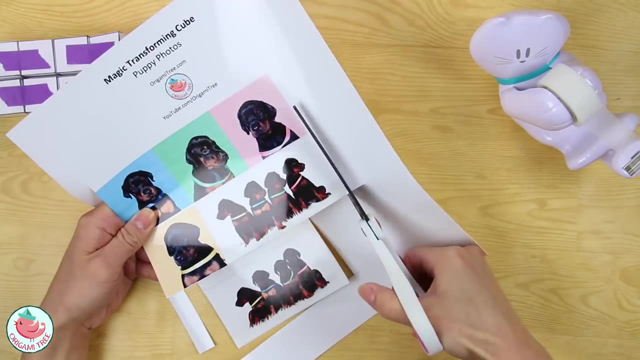 So now that everything is taped down, I'm going to flip it back to the purple side again, where we started. Now we're going to cut out all of our photos. Of course, I'm using the puppies from my template, but you don't have to use puppy pictures if 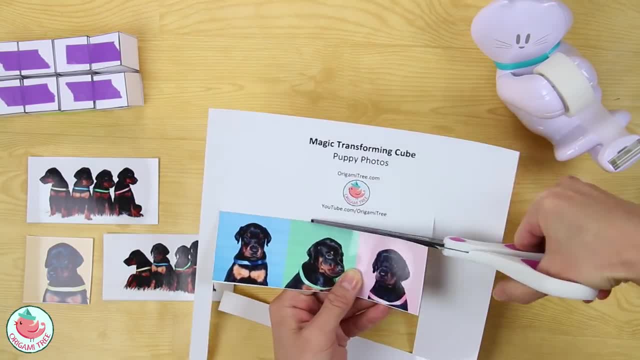 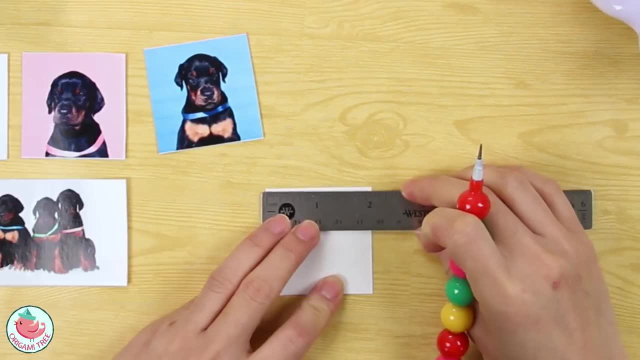 you don't want to, You can always print out your own pictures as well. So now I'm just taking my square photo, which is two inches by two inches, and I'm going to mark off the one inch mark, or the center point of all four sides. 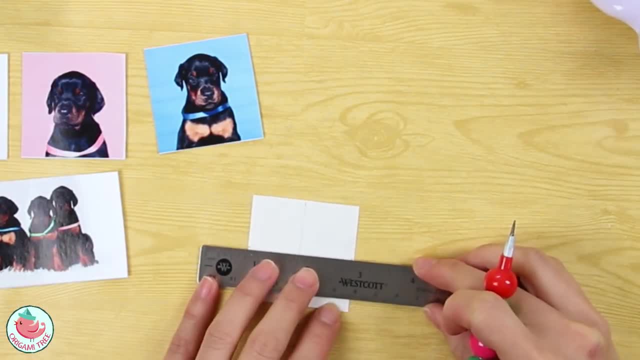 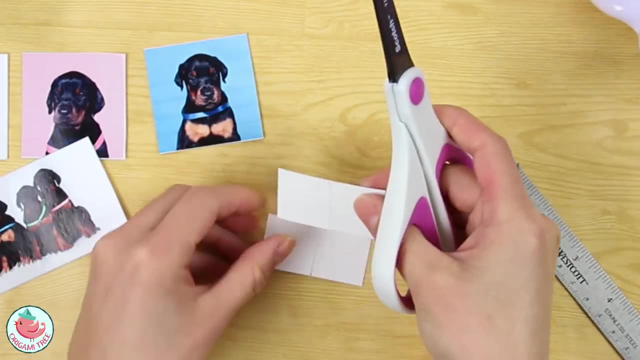 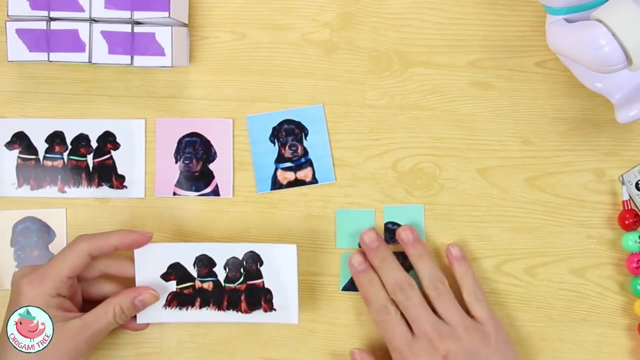 Once I have those center points marked off, I'm going to draw a line across the center points to create an X, And then I'm going to take my pair of scissors and cut the entire square photo into fourths. Now I'm going to move on to the rectangular photos. 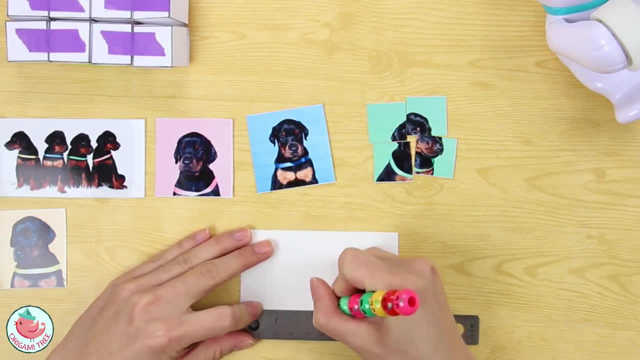 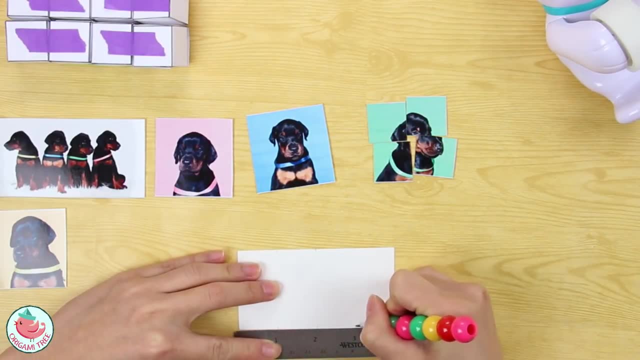 And for the rectangular photos. I'm going to use my pencil For the rectangular photos. they are two inches by four inches, so I will be splitting these into eight equal parts, And so I'm just taking my ruler now and marking off the one inch points on the long side and 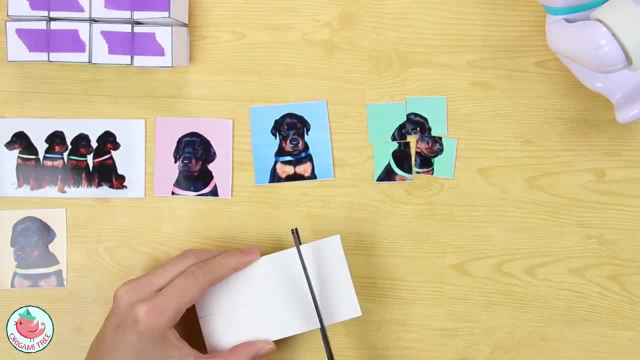 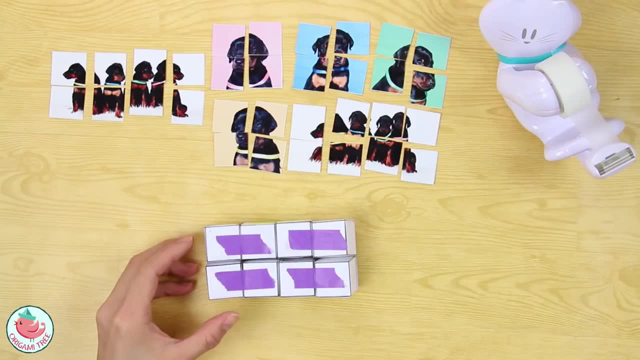 also the short side, and then cutting it into eighths, And once you have all of your photos cut into one inch squares, it is time to stick them onto the magic cube, And so I like to use glue dots, because there is no drying time. 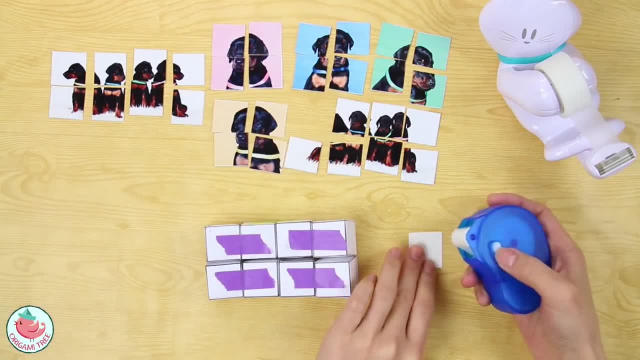 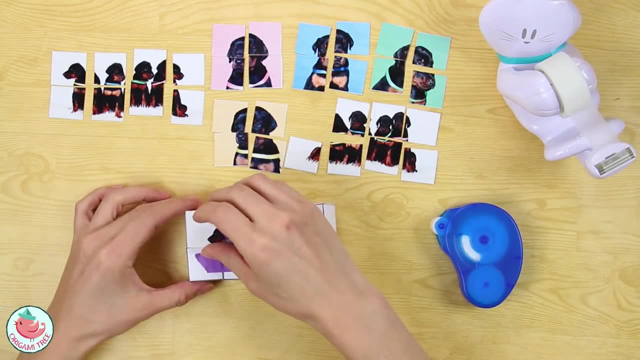 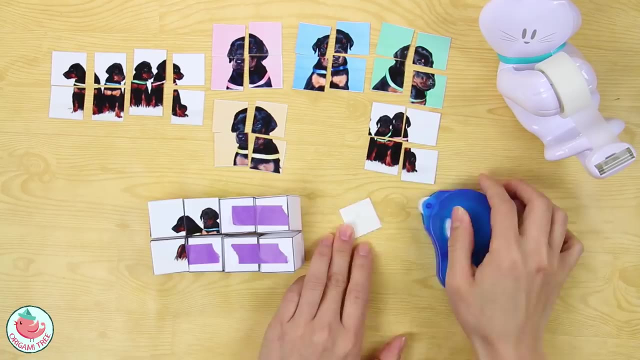 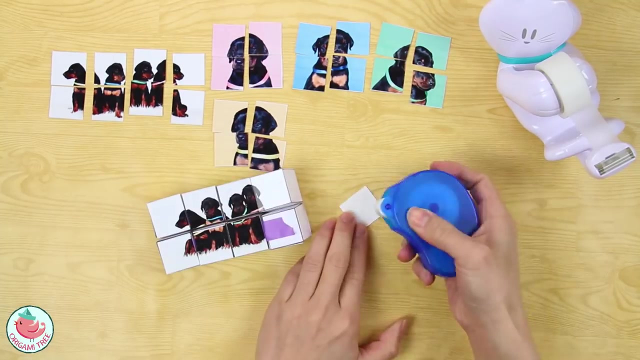 But you can use double sided tape or glue stick, whatever you prefer. So, taking one square from the photo at a time, you're going to glue it onto the corresponding cube on your transforming cube. Now that I'm done with the purple side, I'm going to flip the entire thing around. 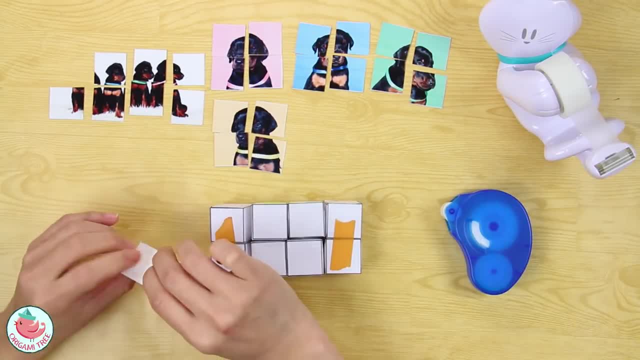 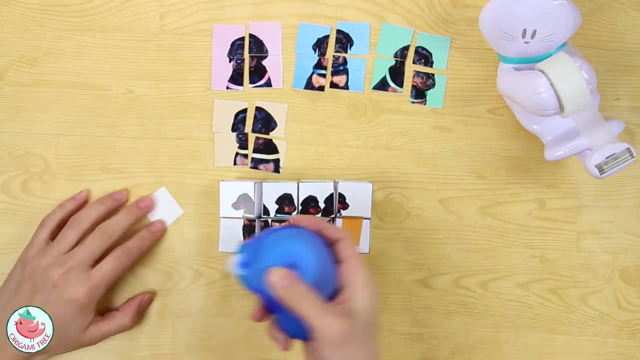 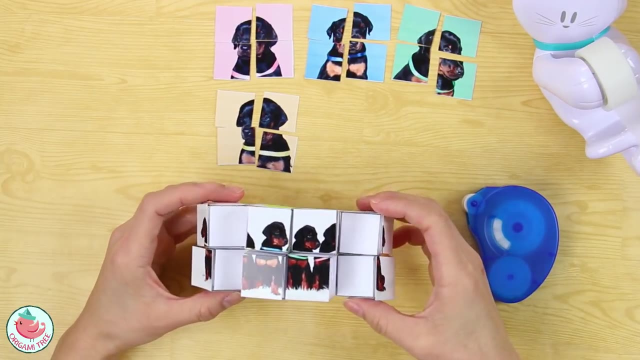 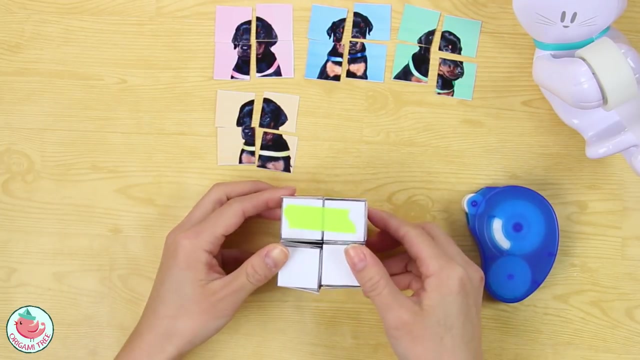 and work on the orange side. Now I'm taking the left and right sides and I am folding them back and under and once you do that, you have four empty sides on the side of the cube and that corresponds to the four pictures that you see on the screen. 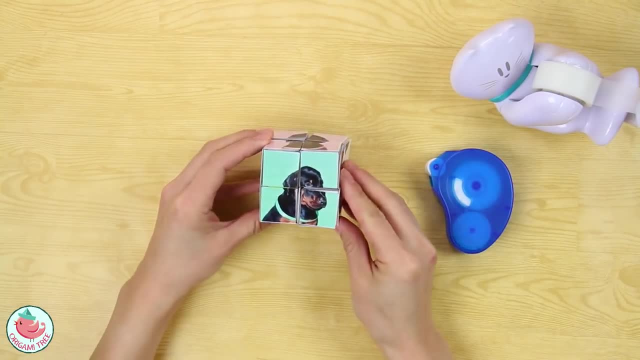 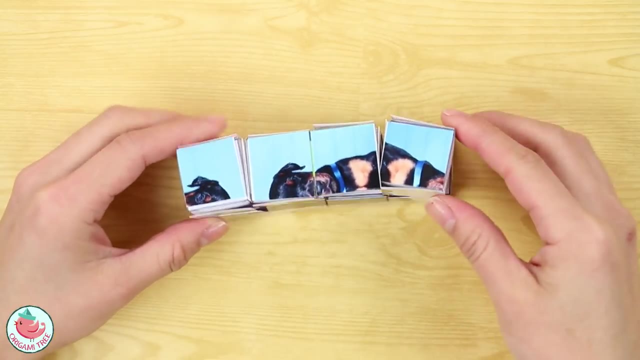 Once you've glued on the last piece of that photo, you're going to flip it back to the way that it was before, which is with the dog with the blue background. I'm going to open it up, swing it over to the side, flip it and then flip it again. 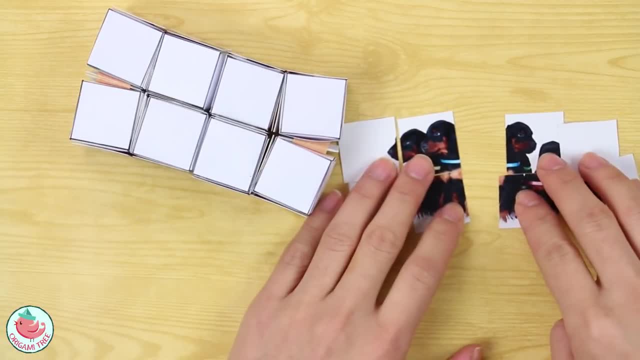 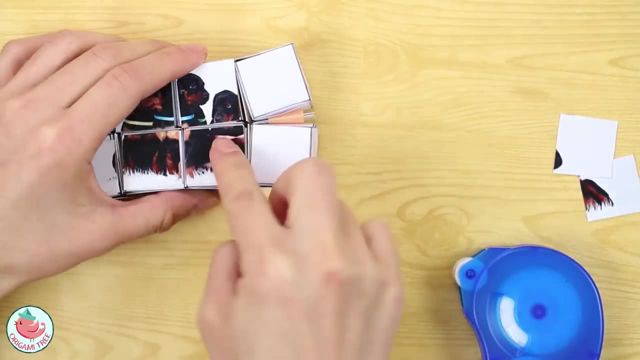 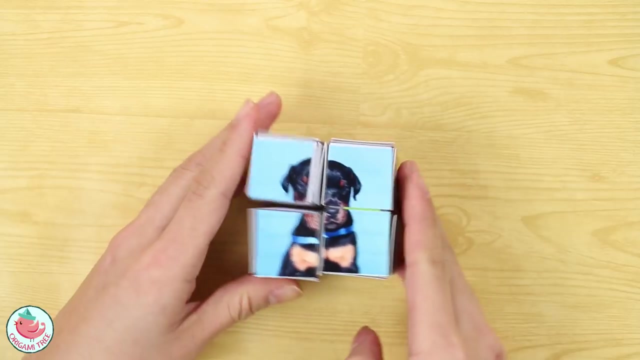 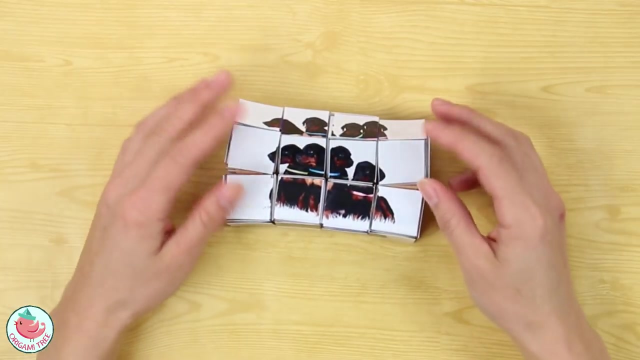 to reveal the other side. I'm going to reveal eight more empty squares and we're going to grab our rectangular picture and then stick it on Now, starting with that dog with the blue background. again, you're going to open it up to reveal the rectangular picture. flip it over again to reveal the next. 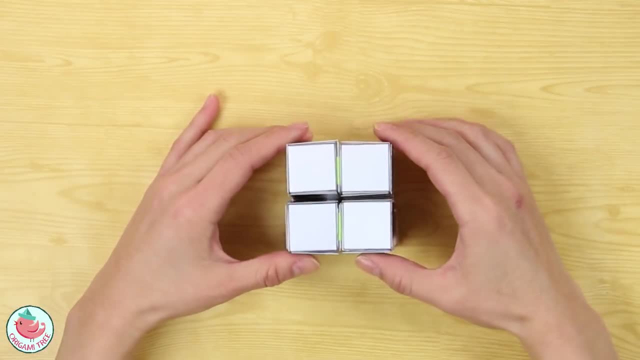 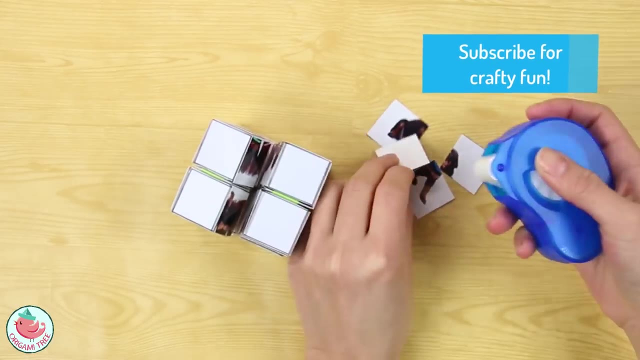 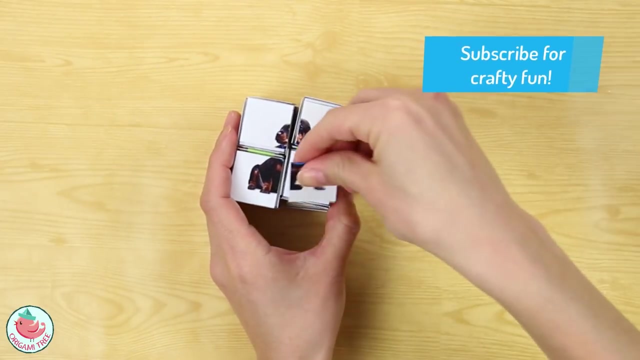 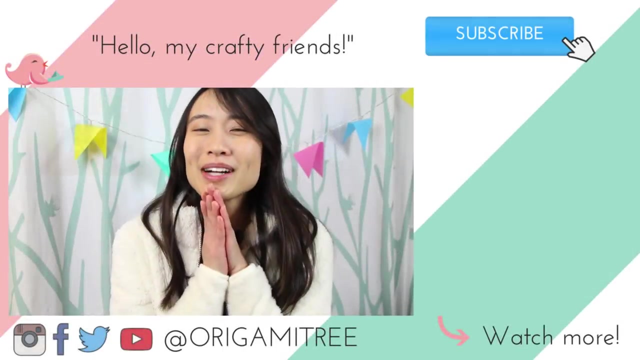 rectangular picture and then open it up to reveal the four empty squares Which are going to correspond to your final square photo. Once you've glued on that last piece of your last photo onto the magic cube, you are completely done. Thank you so much for watching and for sticking until the very end of the video. 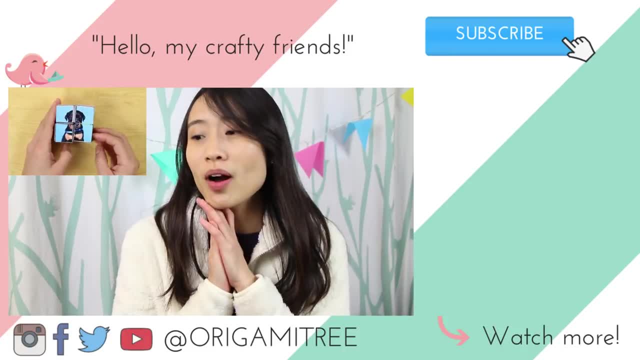 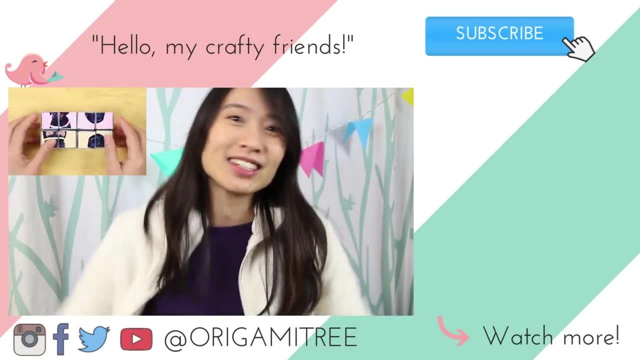 I always appreciate that. Again, I wanted to wish you all a happy new year. Thank you so much for joining me in 2017.. And thank you so much for being here today watching in 2018.. Anyway, I've got to go now, so I'm going to turn off the camera. 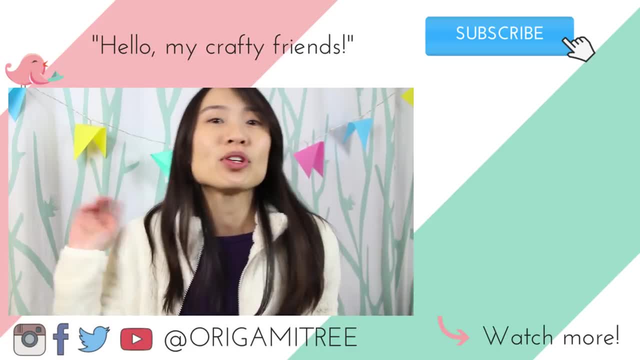 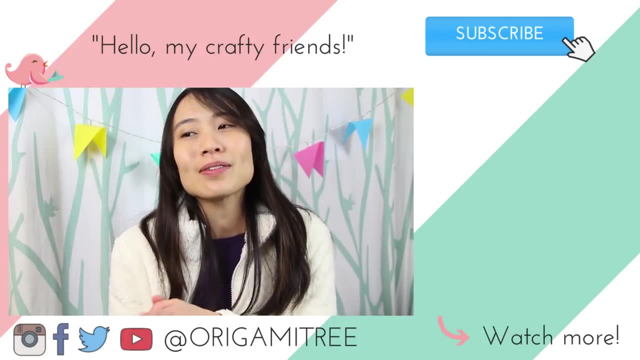 But before I sign off, before you click away, be sure you leave that comment below letting me know what you'd like to see next. Do you want to see more magic cubes Like: should I make a cat one too? I feel like I have to make a cat one because I made a dog one.